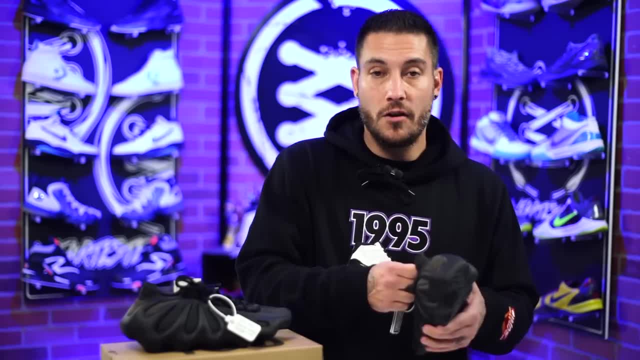 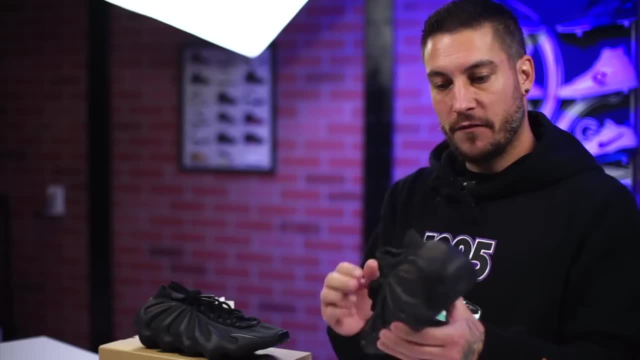 OG of the sneaker reseller. They sell stuff. They've been around for a long ass time, so if you have not purchased from them, you can just know. rest assured that their stuff is authentic. The shoe is so weird It's like folding into itself. I've only seen these once on someone's feet and they were weird. It wasn't this. 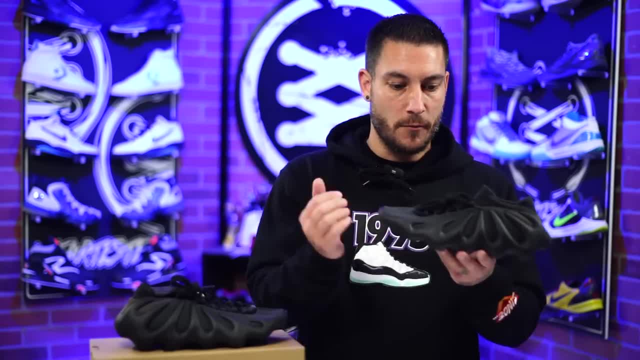 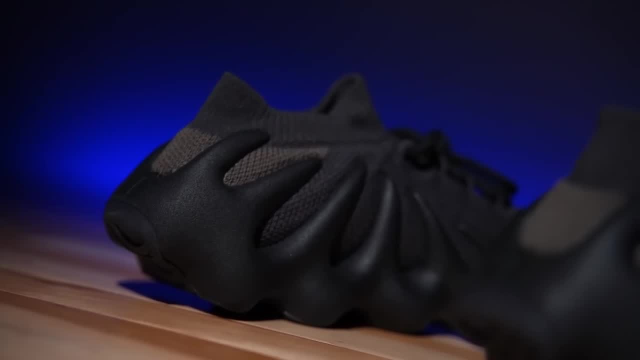 colorway. You were with me, It was the other one. They were like tan and white. Those ones, I think, look a little bit better, but that's not saying much. It's like putting lipstick on a pig, as our friend Brian would say. So it's just like it is what it is. I do think that the shoe, though. 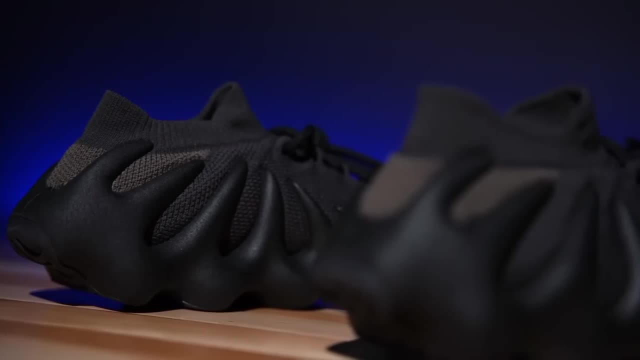 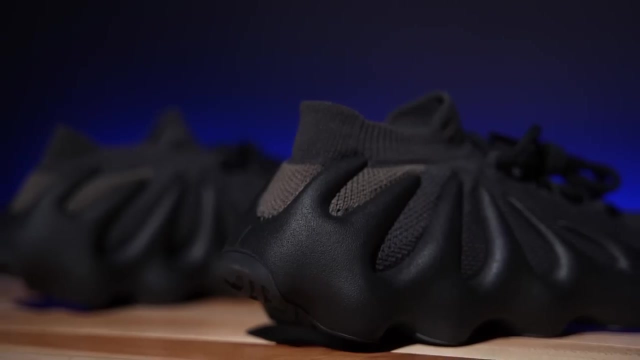 is very interesting, which is what all of the Yeezy stuff, at least current kind of like, gives me, that vibe where it's like, oh, those are hideous, but they're very interesting. as far as footwear is concerned, How it's manufactured, How it's made, It seems like this: 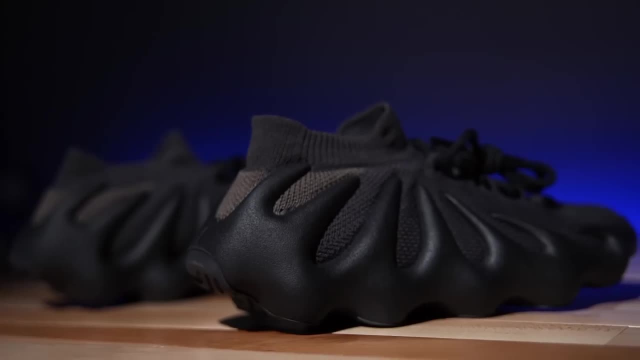 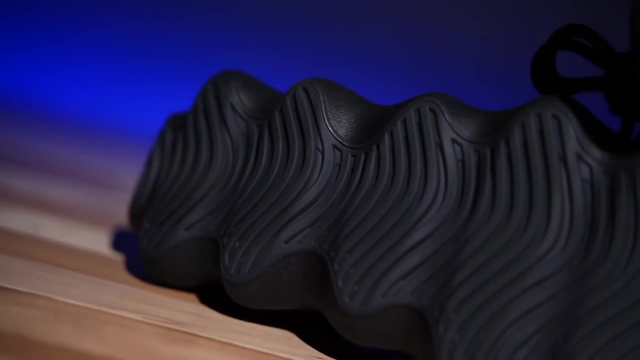 is the stuff that is kind of pushing the envelope, and I think it's interesting They're not just pushing the envelope as far as manufacturing goes, but also design and style. So first things first. we do have a rubber outsole right here. It's kind of got that classic Adidas wave bone pattern to it. 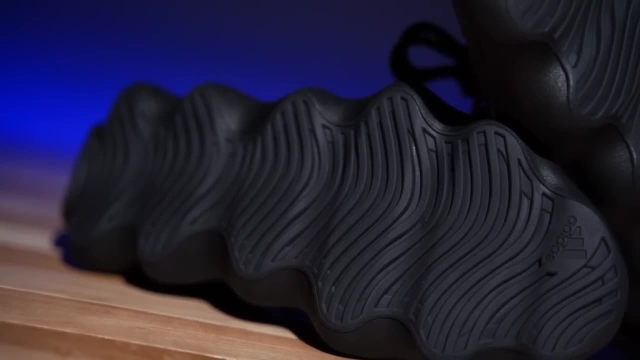 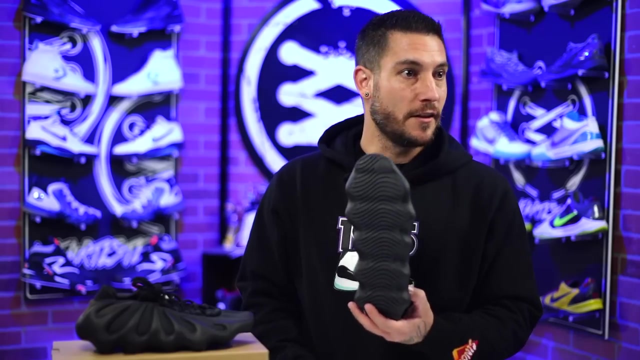 Stuff that we've seen first introduced on the Adidas shell toes or the superstars, whatever it is that you want to call them- Then adopted by, you know, Nike. They stole it and changed it up a little bit and started calling it herringbone, But this thing right here, man is so. it's so weird and 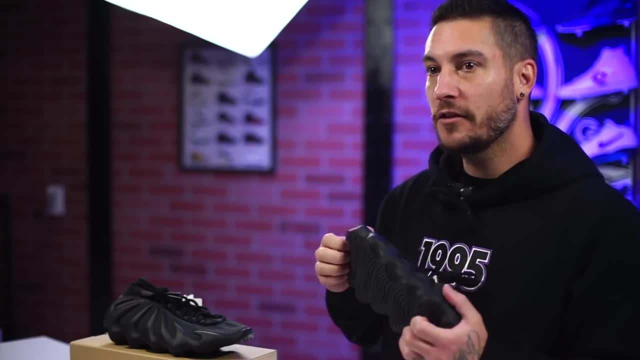 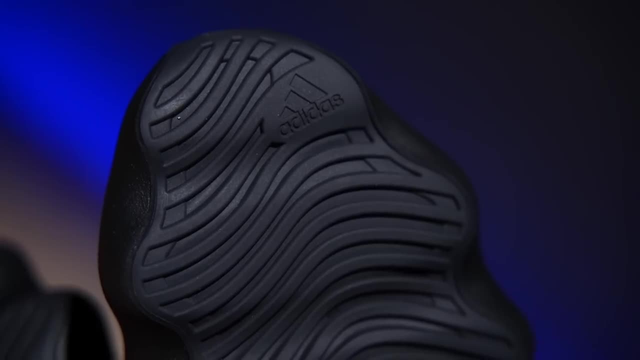 flexible and all that stuff. The rubber feels strange, like it doesn't feel like traditional rubber. I feel that it's almost like slick. It's very interesting. So it is one piece. I don't know really what to say about it other than it is what it is. But the main portion of the shoe is the 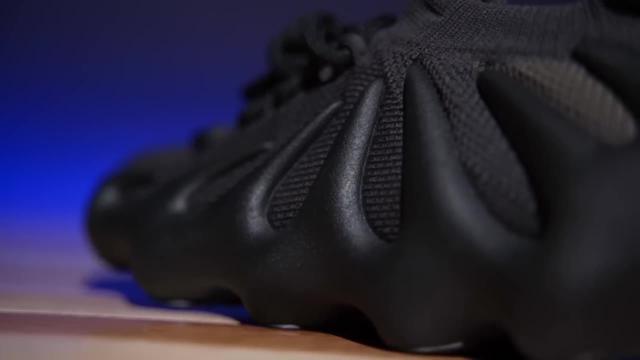 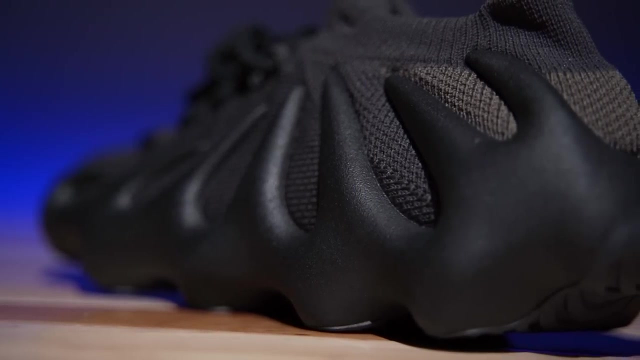 upper and this thing that cradles it, The thing is the midsole. Does it remind you of anything? Venom, Venom, really, Yeah, Oh, okay, I guess it does To me. it reminded me of Beetlejuice when they're in the house and that sculpture thing that like. 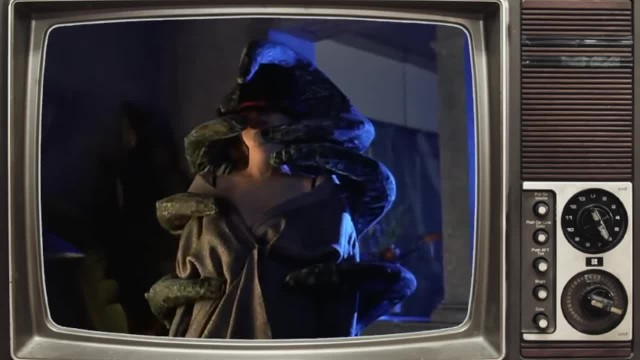 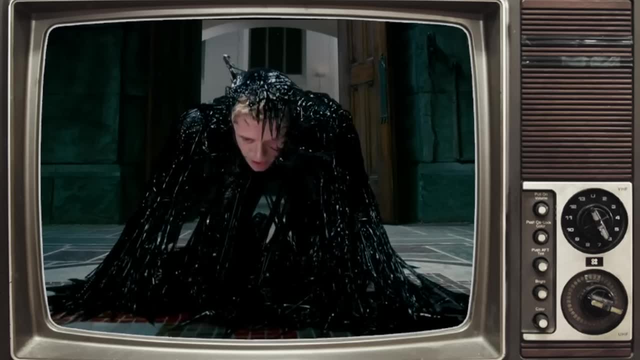 her artwork. Yeah, and it like what this thing looks like. Like it's just gonna like grab your foot. Oh no, it looks like the symbiote, like crawling up. I do agree with that a little bit. That actually would be really cool. You know how they did the. 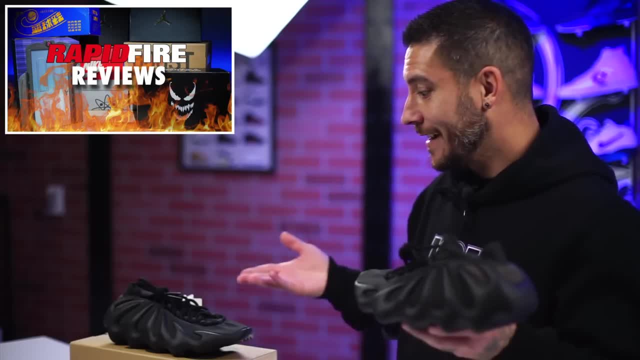 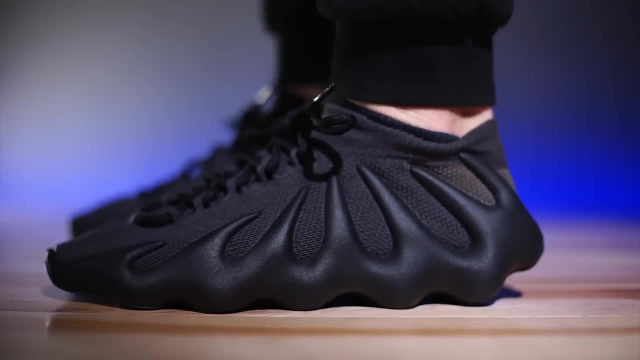 the Dawn. issue three: Venom, and this would have been a great candidate for that, but I don't work with, Anyways, this whole midfoot midsole cage. whatever this is, it's all one piece. This is actually EVA, so I thought that you know. 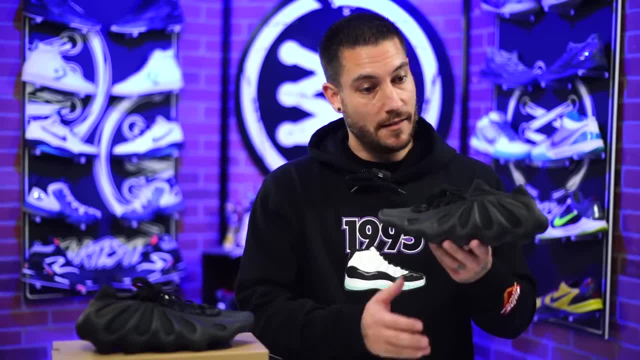 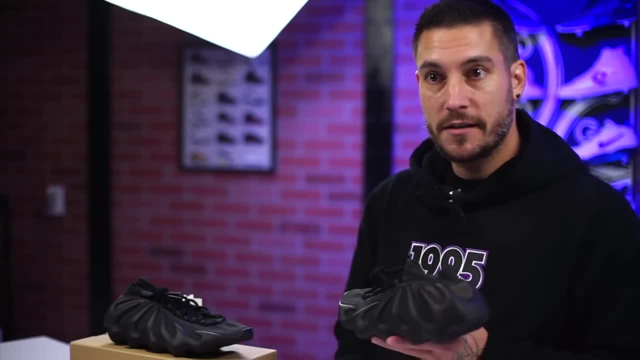 they might have gone the boost route and all that stuff, What they've done in the past. they started off with boost, with the 750s, the 350s, the 350 v2s, so on and so forth, The 700s, and yada, yada, yada. 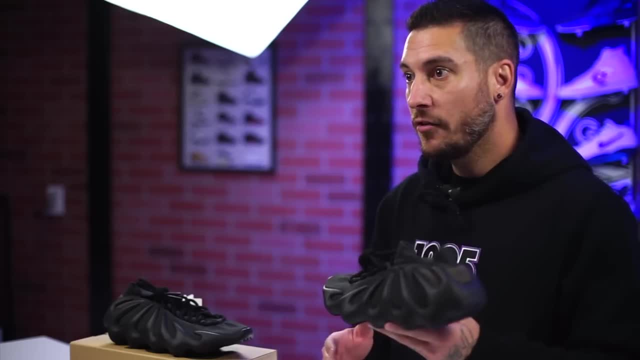 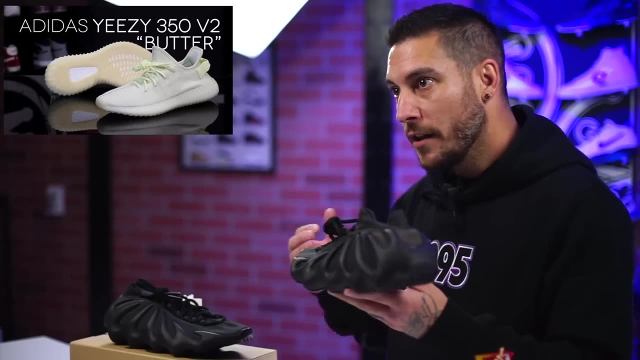 These are different, though. This is just a basic setup. It's not anything crazy. If anything, these kind of remind me of what Kanye started with back in the day, which was the 350, but a new version of it, So like there was the. 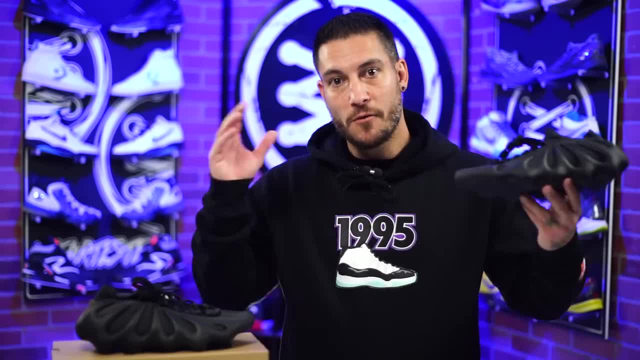 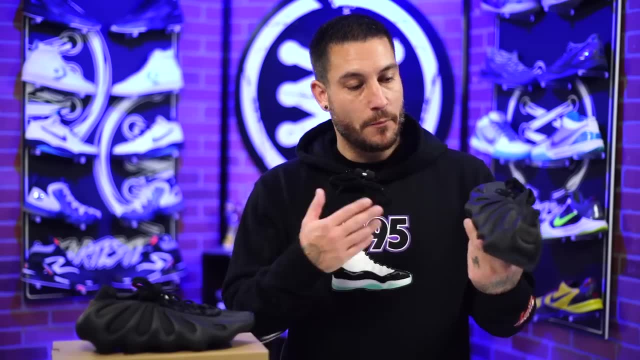 Roshi run or the Rosh one from Nike, and everybody was going mad, crazy over those. and then Kanye made the 350 and was like, oh, we're gonna make this and make it cooler, more comfortable. This feels like kind of like going back to that basic version of the Rosh and yeah, so it just seems like a new gen. 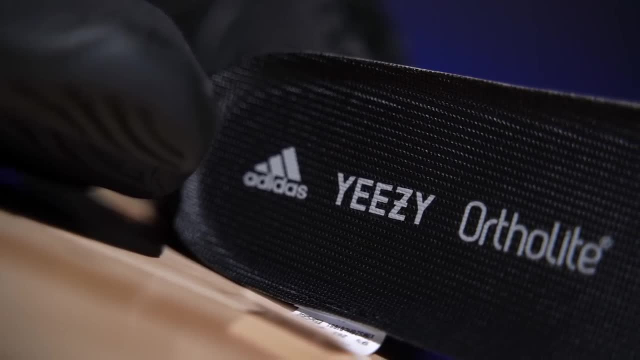 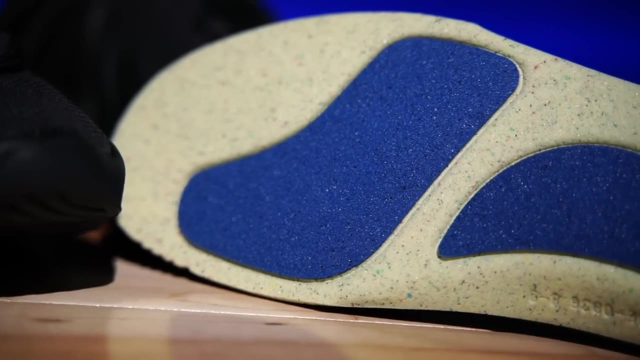 sock shoe, which is interesting. Now the cushion comes from this bad boy right here, This insole. it is ortholite, It says so right there on the top, but it's got a bunch of different little pads of different density foams and things like that. so I do like it. I think it's pretty cool. 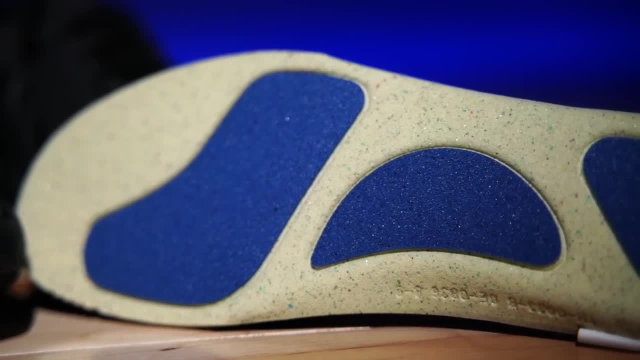 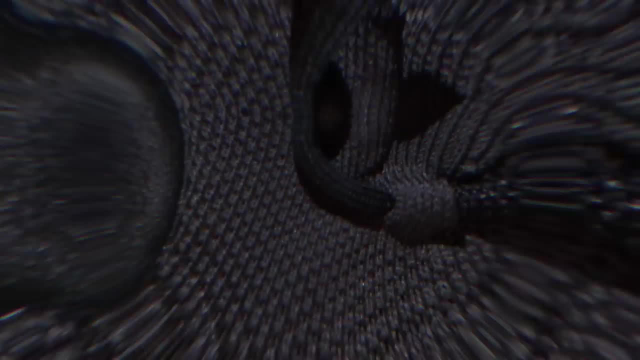 Reminds me of the Air Jordan 14s. The insole is completely removable. if you were interested in grabbing a pair of these and you need orthotics or whatever you need some arch support, you can go ahead and throw that in there and it'll fit just fine. Now the main section of the shoe is: 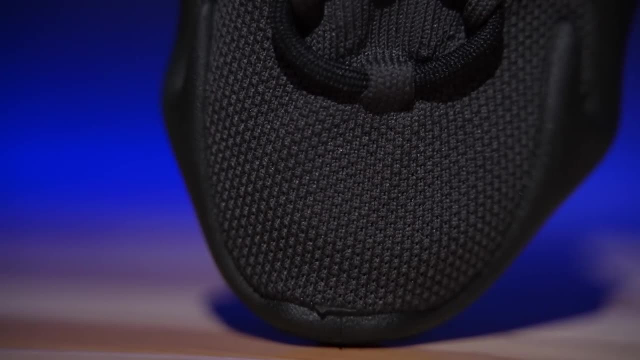 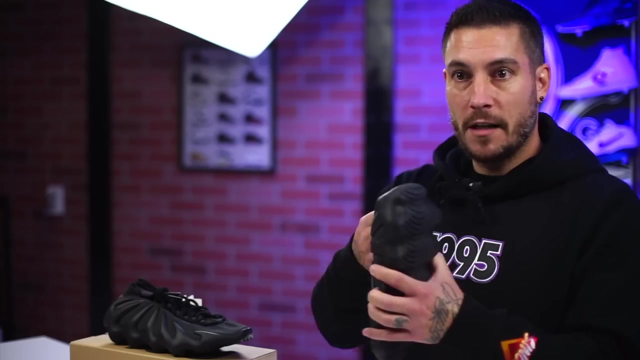 the upper. The upper is all knit everything. This is the part where it's like real weird, like the way that they've constructed this shoe being fully knit. there's nothing reinforcing it. There's no heel counter. I mean there's a little. there's like a little shape back there. that's the. 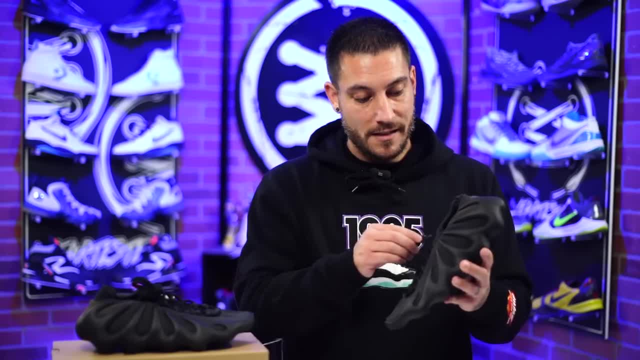 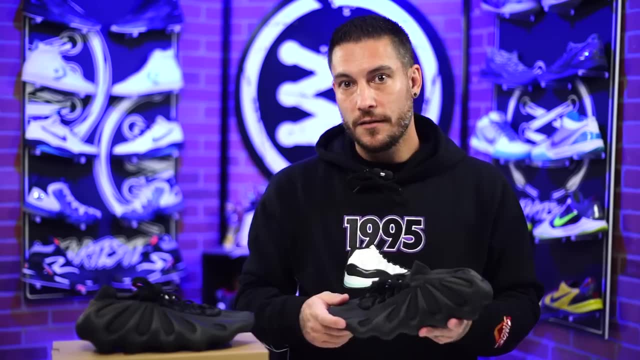 heel, but it's not anything crazy. It's a water shoe Kind of. I mean, it's not neoprene, it's all knit, but like it's just really weird, like even the eyelets are knit. It's like somebody sat there and crocheted this and they were just like, yeah, this is all we can do. I don't know what to think about. 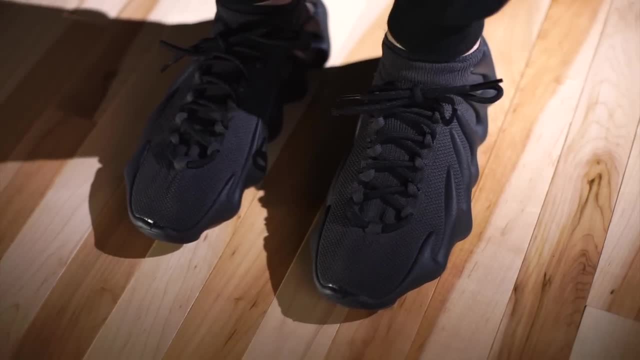 this. I don't hate it, I don't love it, I would never wear it. It's weird like they kind of remind me of the foam closet, like it's like that type of weird The foams like, even when you look at them. 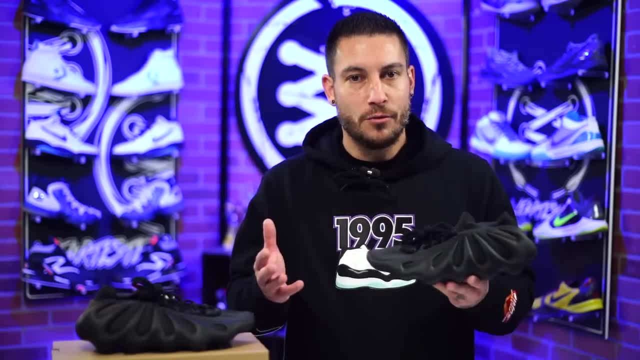 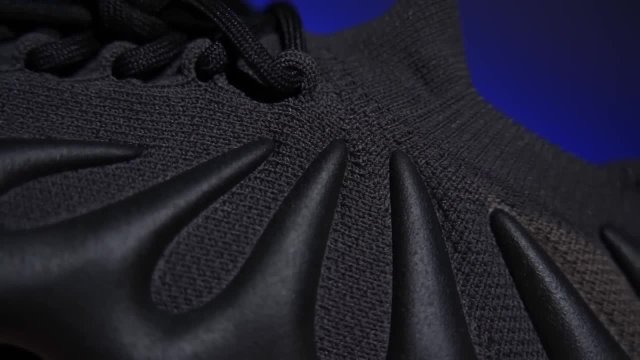 still. granted, they've been around since what? 97.. It's a shoe that you look at still in 2021, and you're like: what the f**k were they thinking? What the f**k are they smoking? This is that shoe, but for now, Modern tech and stuff like that, like 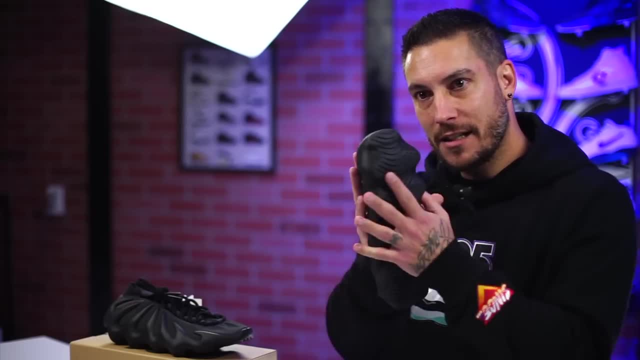 there's an internal midsole inside of the sock and it's all clamped together to this EVA midsole. It's so strange. It's the weirdest of our time. I do think that the foam closet is weirder, but that's. 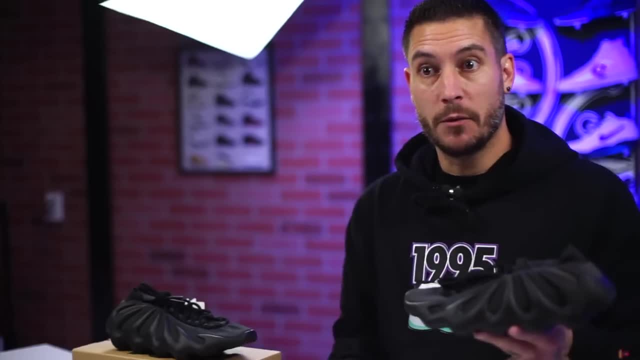 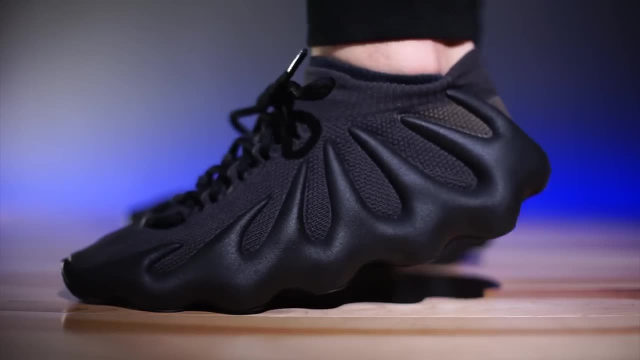 from a different perspective, That's, from a manufacturing perspective, which is like liquid foam. Now, as far as sizing is concerned, these are actually not my true size. I'm usually a size nine. These are a size nine and a half and they fit perfect. They fit one to one. They fit like my. 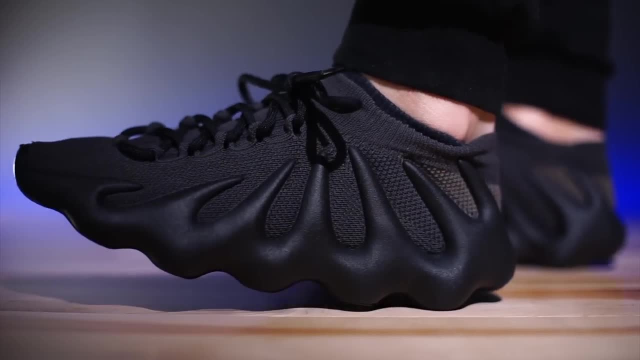 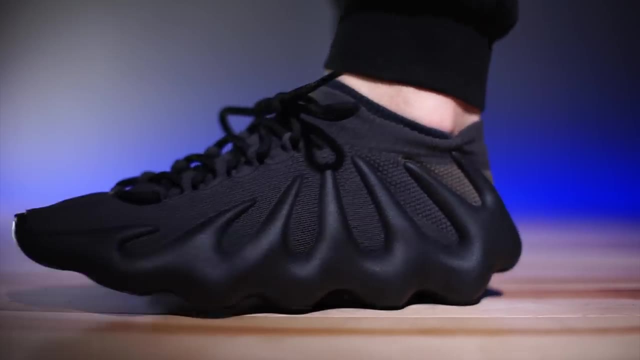 socks, but it's a shoe and uh, yeah, it's really, really weird. So going up half a size would be probably recommended. Could you go true to size, I believe. so I think the upper is so forgiving that it'll be fine. Do you feel all of the symbiote stuff? 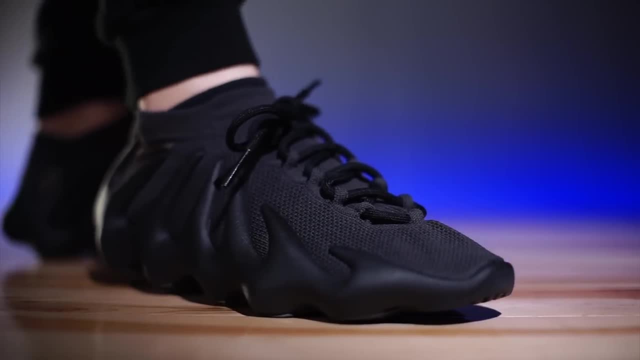 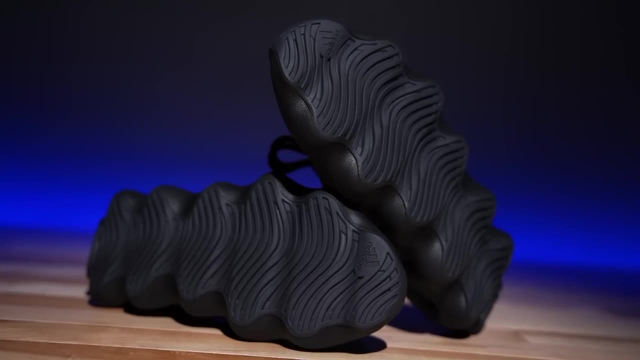 No, you don't. That's something that I actually think is quite surprising. It does hug the foot in like such a perfect way that they are actually really comfortable. So yeah, even the waves that are on the bottom, like I don't know how well you can see it, but there's, like these, like you know. 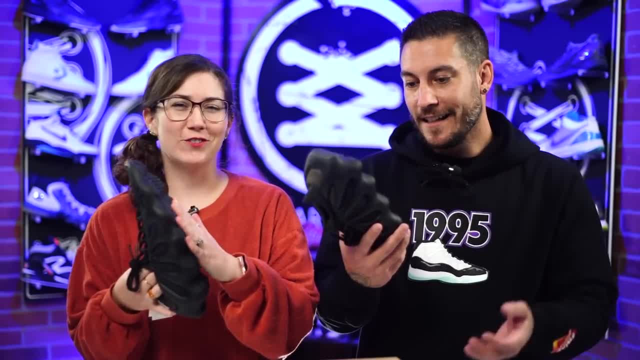 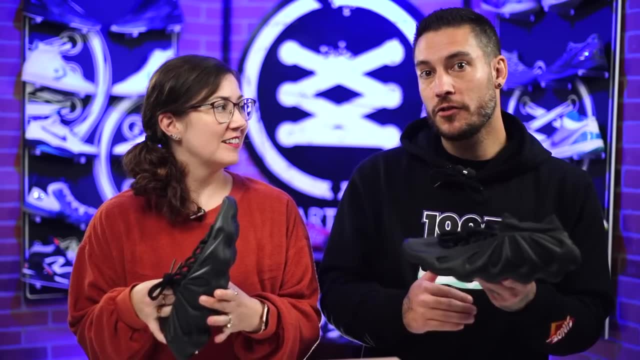 looks like a ruffles chip. It's like a crinkle cut, Yeah, and it's so interesting that it's the design aspect of all of these things put together that makes them so functional and so comfortable, despite the design itself being so wild and out there Even though they look jarring. it's one of 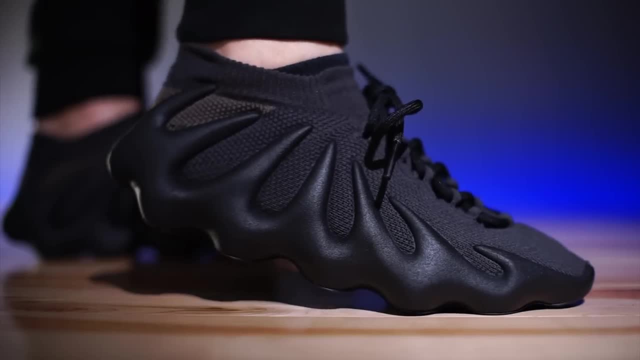 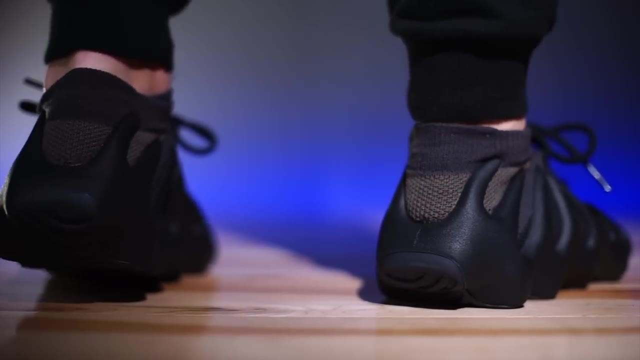 those things where it's like, no, they're not that bad. Yeah, it's kind of like the person wanted something that felt like they were wearing nothing but that their foot was fully protected. at all times, I agree, like especially in this colorway, I feel like I'm a ninja- Oh, a fellow chucker, eh. 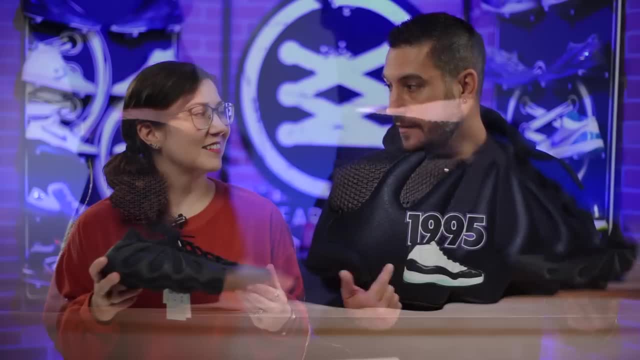 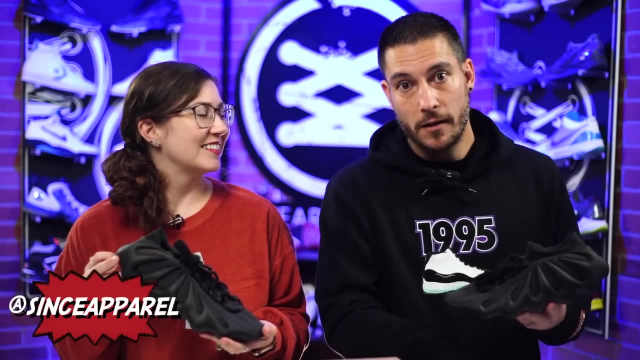 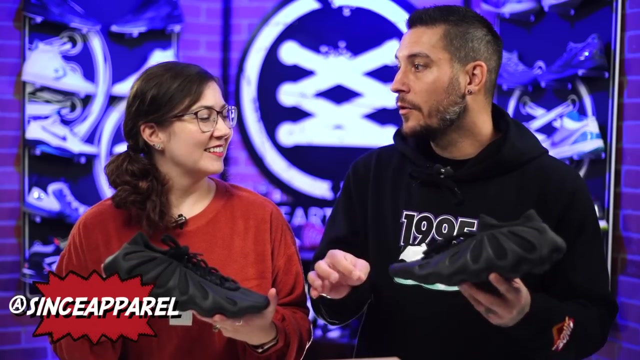 I'm silent, Comfortable. Also, these come out very soon, November 11th This week, okay. so if you are not following Sense, Apparel on Instagram. if you are not signed up to the newsletter, you're probably going to miss out. I think this is the one where I'm not going to post it on the YouTube channel. 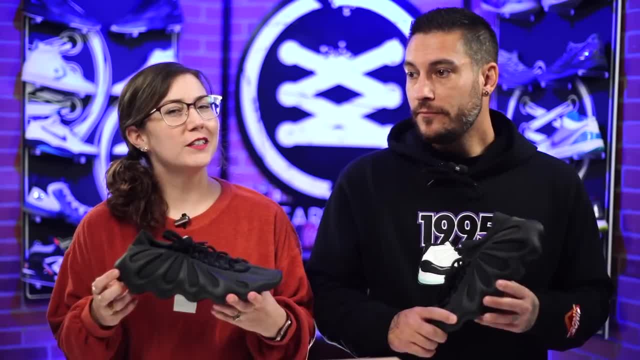 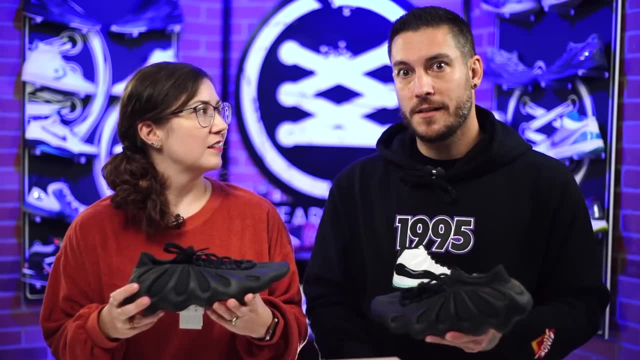 as far as like what do they call it? the community tab? Yeah, the community tab is very hit or miss. It's super hit or miss. Half the time we just get angry comments being like I just saw this and it's like eight days later or whatever, and I'm just like bro, like I don't. 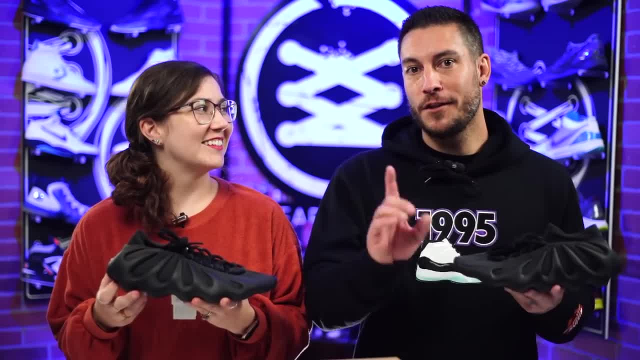 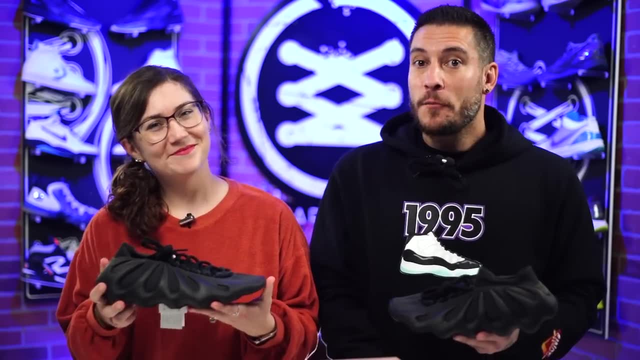 design like the algorithm, you know what I mean- like it's based off of what you watch, so like, if you don't watch us every day, then it's not going to show you our stuff and then you're going to miss out, even though I talk about this in every video. so I can't really help you, but they will.